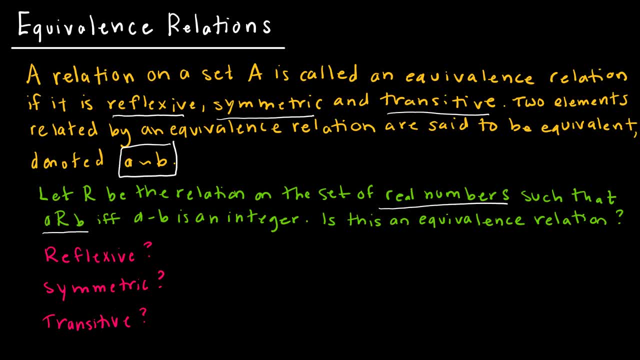 real number and we're saying that a is related to b if, and only if, a minus b is an integer. So is this an equivalence relation? So we'll start with the easiest property, which is the reflexive property. We're saying a minus a, So if a is related to a, that implies that a minus a is an integer. Well, we all know that a minus a is zero, no matter what a is, a minus itself is zero, And so 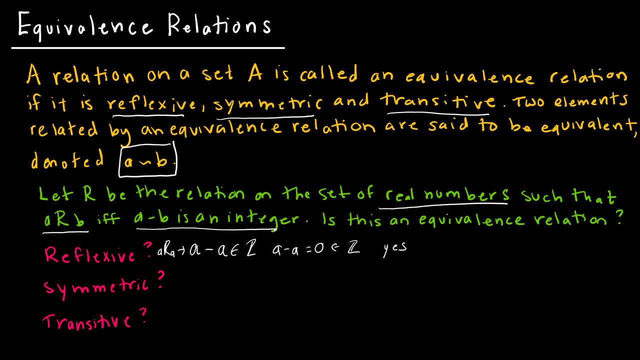 zero is in fact an integer. So yes, this is reflexive. Is this symmetric? So symmetric says: if a is related to b, that implies that b is related to a. So is this true? So if I took a minus b and got an integer, that's implied Will. is it true then? 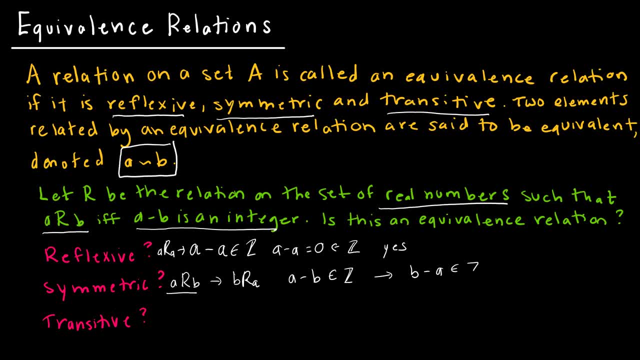 does it imply that b minus a is an integer as well? Well, absolutely, that is true. So think of it this way: Let's call a minus b, we'll say that's c, And we know that it's an integer because it tells that's the hypothesis in the implication. So this is true: a minus b is equal to c, which means if I took b minus a, what am I going to get? The opposite sign of c, unless, of course, c was zero. then I would still get zero. 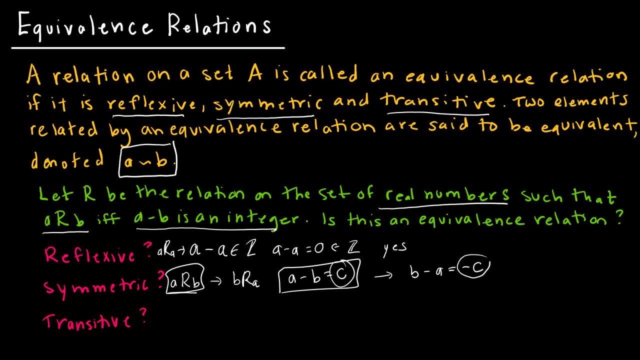 And we know that if c is an integer, then the opposite of c is also an integer. So, yes, this is symmetric. So now let's look at the last one. Is it transitive? That's the hardest one. And that one again says: if a is related to b and b is related to c, it implies that a is related to c. Oops, I think I used an a here on accident. A is related to b. 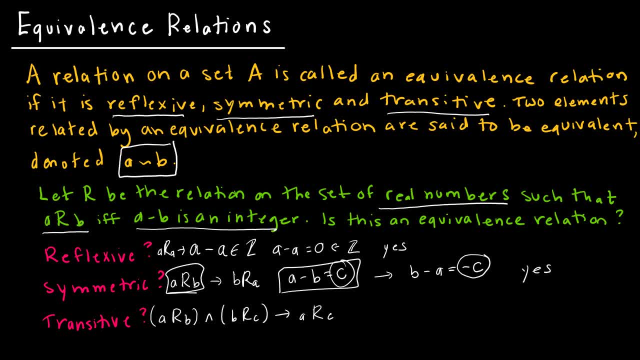 So the question is: is that true Because a is related to c? says that a minus c must be an integer. Well, this one says a minus b is an integer And this one says b minus c is an integer. So this is kind of a tricky way to go about it, But we're going to say a minus c is the same, An equivalent way to write that is a minus b plus c. 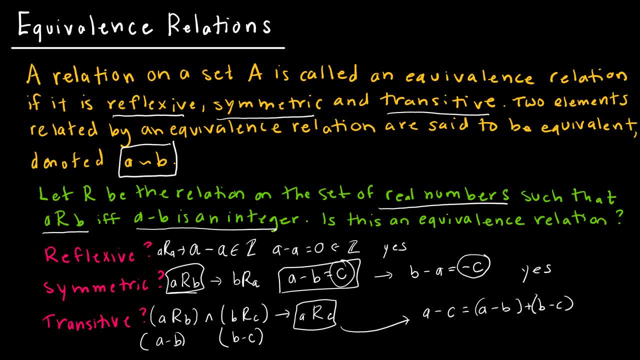 Now, I know this is an integer, And I know that this is an integer, And a minus b plus b minus c gives me a minus c. So obviously I didn't break any rules. So then the question is: is this an integer? Well sure, If I take an integer plus an integer, I get another integer. So a minus c is in fact an integer if b is related to c. 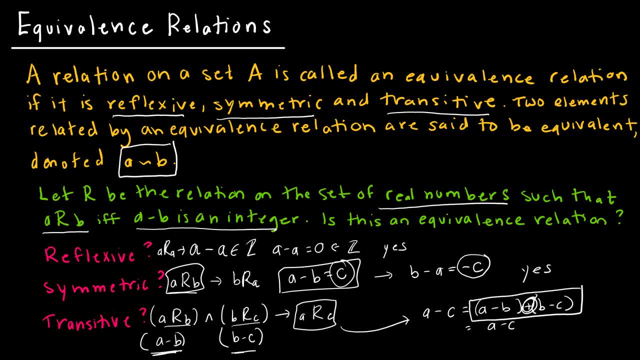 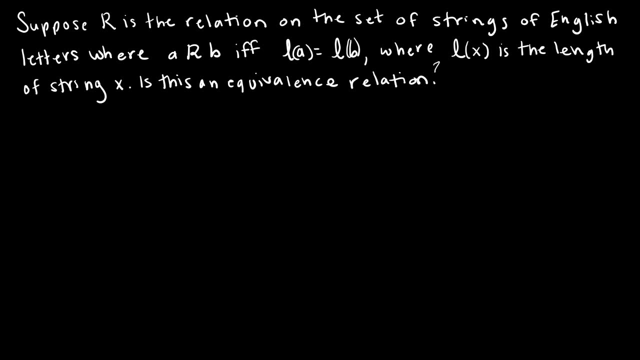 A is related to b and b is related to c, Or in other words, if their differences are integers. So because this relation is reflexive, symmetric and transitive, then the relation is in fact an equivalence relation. Let's take a look at another example Now we have, suppose r is the relation on the set of strings of English letters, where a is related to b, if l of a is equal to l of b, where l of x is the length of string x. 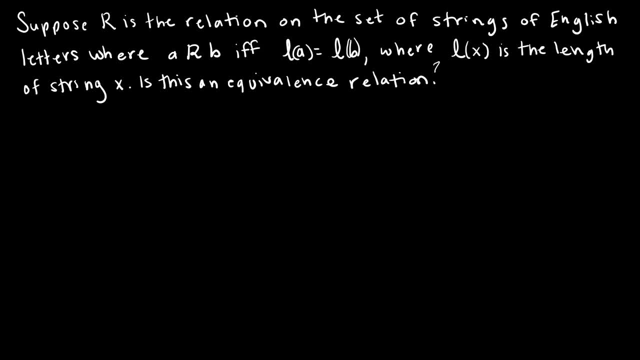 Thereafter, if a is related to b, then the relation is in fact an equivalence relation. So of course we're going to have to check the properties again. We'll start by checking reflexive, And reflexive, remember, means a is related to a. 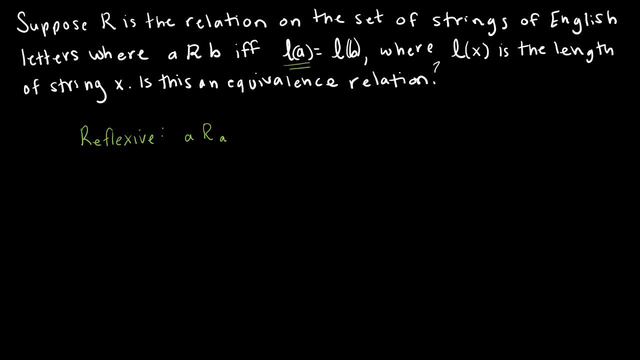 So is it true that the number of letters in the word of a is equal to the number of letters in the word a? Sure, So if the word is cat, then l of cat is 3.. Then of course, 3 equals 3.. 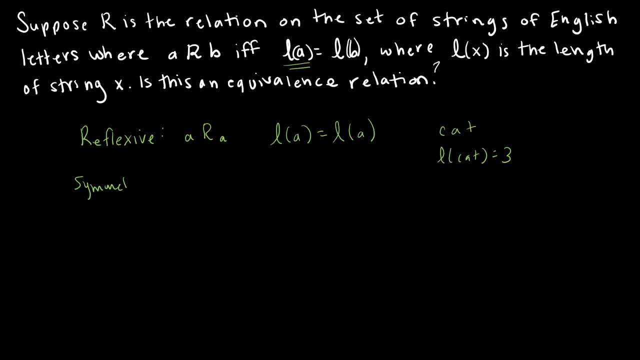 So now let's look at symmetric Symmetric says: if a is related to b, then b is related to a And again. so I'm sorry, I should have put yes over here. So is that true? Okay? so again let's say l of a is equal to 4.. 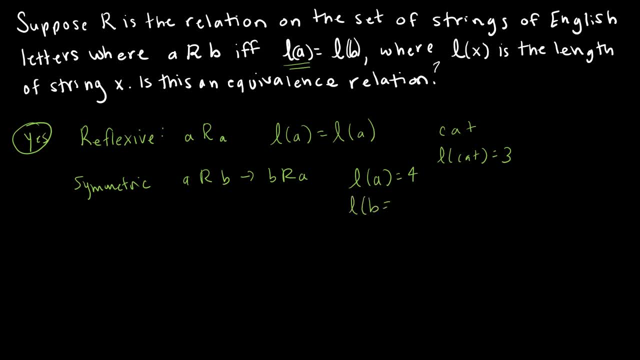 There's four letters. l of b is equal to 4, which means a is related to b, And then is it also true, then, that b must be related to a? Well, if 4 is equal to 4, then 4 must be equal to 4.. 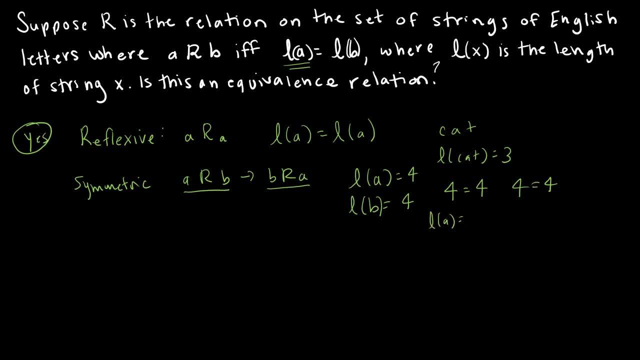 So yes, because l of a is equal to l of b and l of b is equal to l of a. It's always going to be true. Now let's take a look at transitive, And again. transitive says: if a is related to b and b is related to c, it implies then that a is related to c. 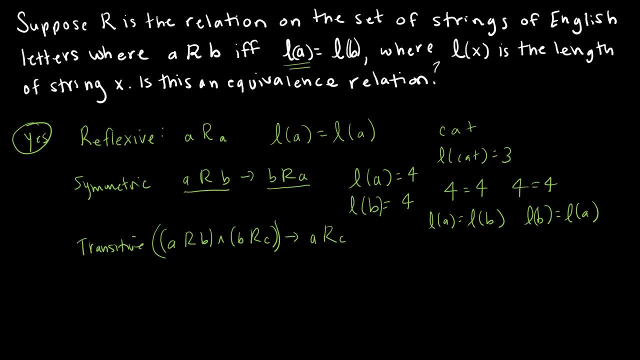 And again, it's not very difficult for us to figure this out. Let's say l of a is l of a is 7, and l of b is 7, and l of c is 7.. So does that make sense then that a is related to b? 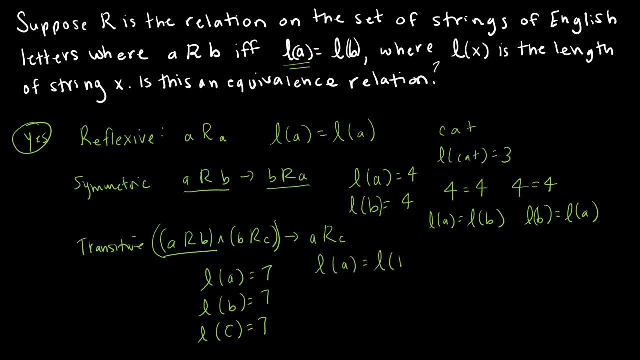 Well, l of a is 7, and that's equal to l of b. so that's true. And l of b is 7, and that's equal to l of c, which is 7, so that's true. So is it true now that a is related to c? 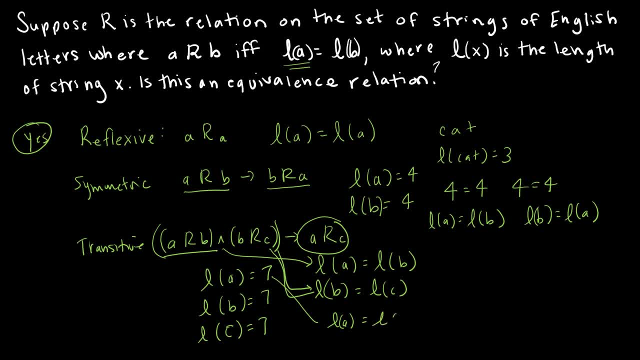 Well, l of b is 7, and l of c is 7.. Well, l of a is 7, and l of c is 7, and so, yes, it is true. So, yes, it's reflective, reflexive, yes, it's symmetric and yes, it is transitive. 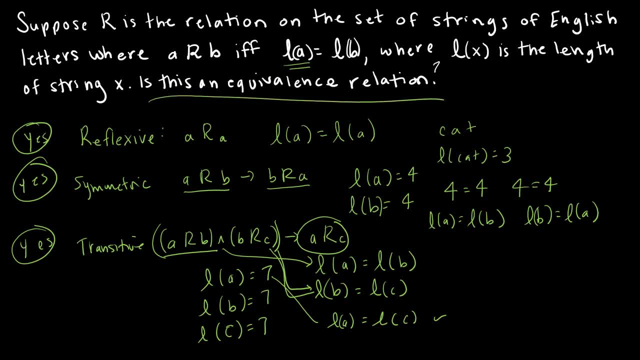 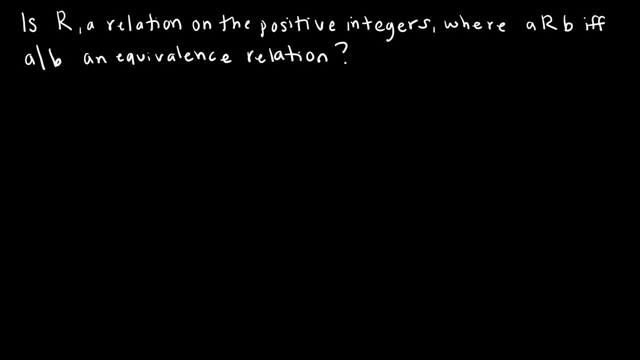 So is this an equivalence relation? Yes, it is. Let's take a look at just one more example We have is r, which is a relation on the positive integers, where a is related to b if, and only if, a divides b. 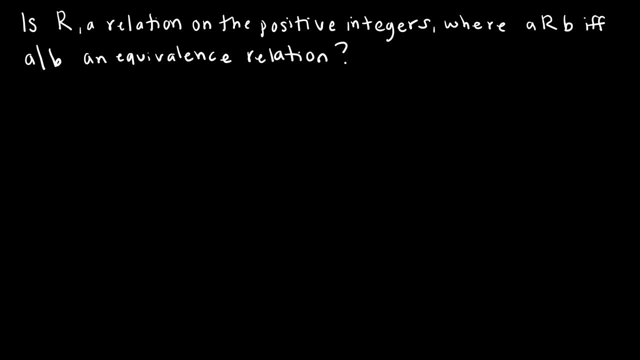 Is that an equivalence relation? So again, let's just recall what it means to say a divides b. It means a goes into b evenly, with no remainder, or b divided by a is an integer. So is this in fact true? 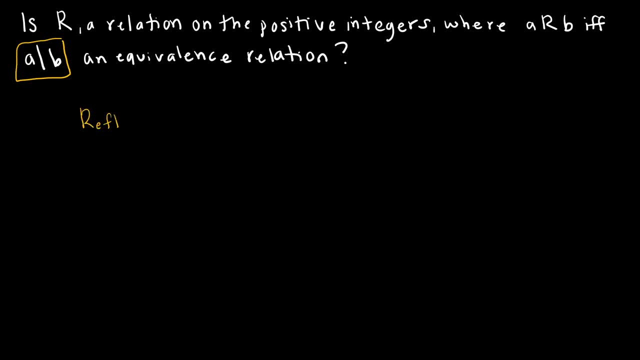 So let's start with the reflexive property. The reflexive property says that a must be related to a. So is it true for all positive integers that a divides itself? Well, I don't even need to show an example, It's very simple to know that that is, in fact, true. 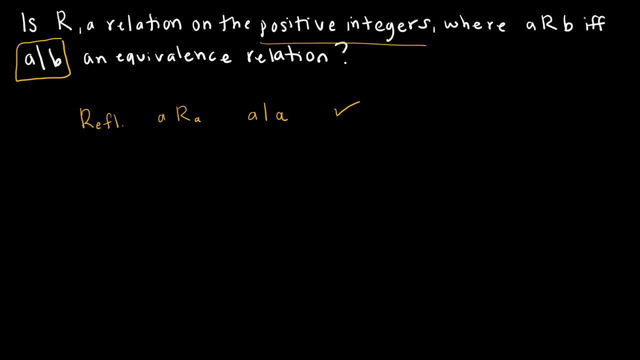 2 divides 2,, 7 divides 7, 13 divides 13,. we get it. Any positive integer is going to divide itself and the quotient is going to be 1.. So, yes, it's reflexive. Is this symmetric? 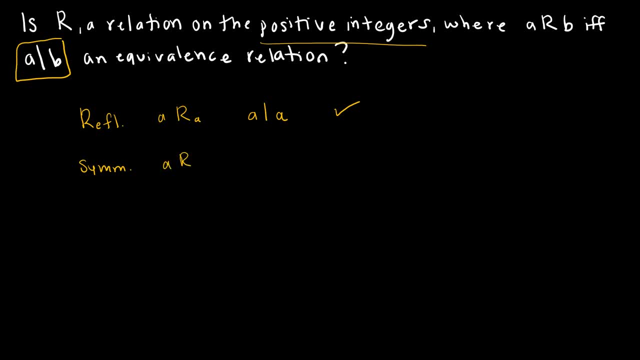 And remember: symmetric says if a is related to b, it must imply that b is related to a. So that tells me, if a divides b, then b, b must divide a. Well, hopefully you can tell just right off the bat that this is not going to be true. 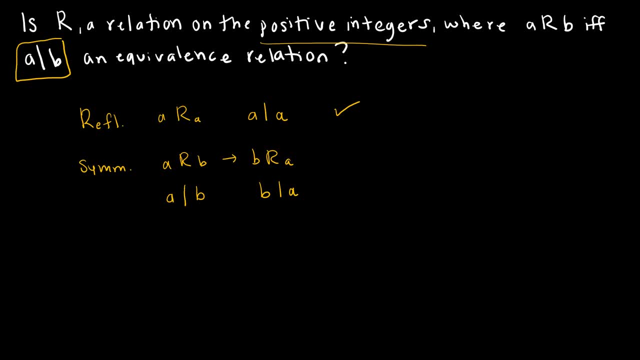 but I can show it fairly quickly with a counterexample, And remember that's all that's required. to show that something's not true is a counterexample. So 2 divides 8, because 2 goes into 8 evenly, with no remainder. 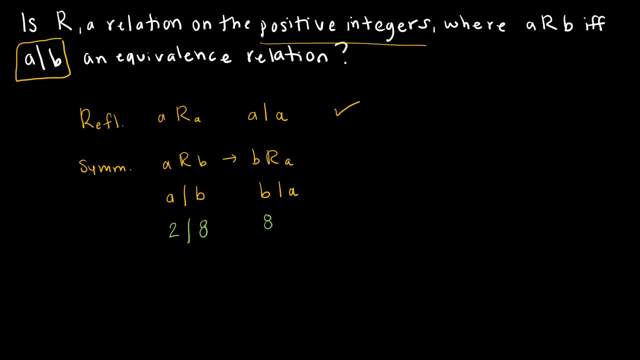 8 divided by 2 is 4.. But does 8 divide 2?? Well, 8 does not go into 2 evenly, because I would in fact not get an integer, I would get a decimal. 8 into 2 is 0.25.. 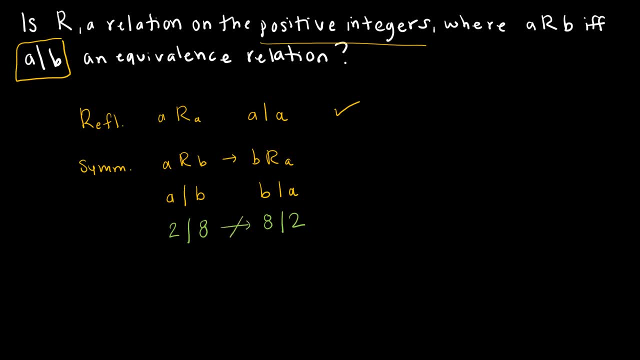 So of course this does not imply this. So this is not symmetric. So do I have to continue to check the transitivity property? I sure don't. I could stop right there, But just for practice we'll go ahead and take a look. 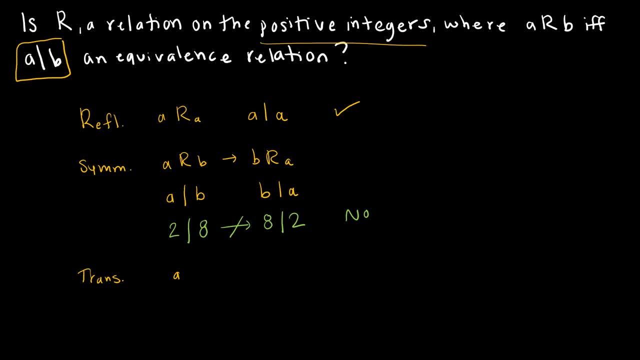 Remember, transitive says So, of course. Sorry, I should be clear. We've already answered this question and the answer is no. it's not because it's not symmetric. But again, let's go ahead and take a look at the transitivity. 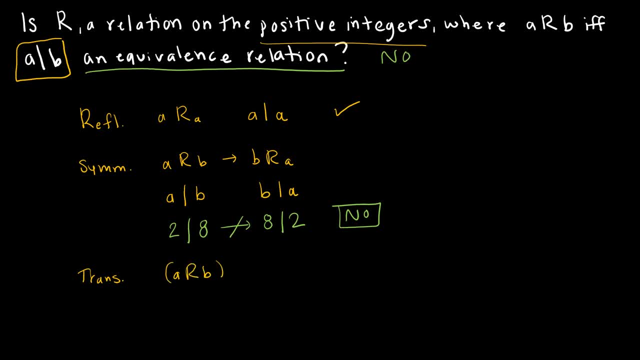 So let's go ahead and take a look at the transitivity property. just for practice, This says: if both A is related to B and B is related to C, it implies that A is related to C, And again, this one should be pretty straightforward. 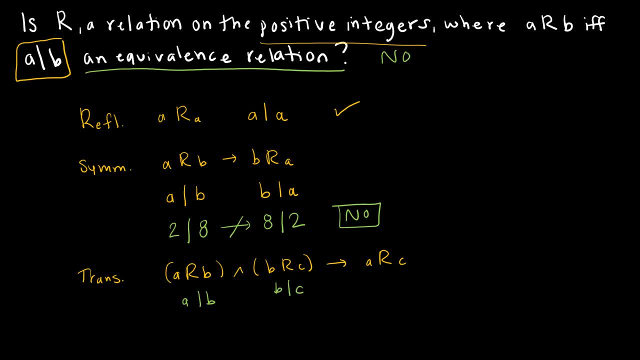 This one's saying A divides B. This one's saying B divides C. Does that imply A divides C? And this one is in fact going to be true? So if I take a look at A divides B, let's just look at an example using actual numbers. 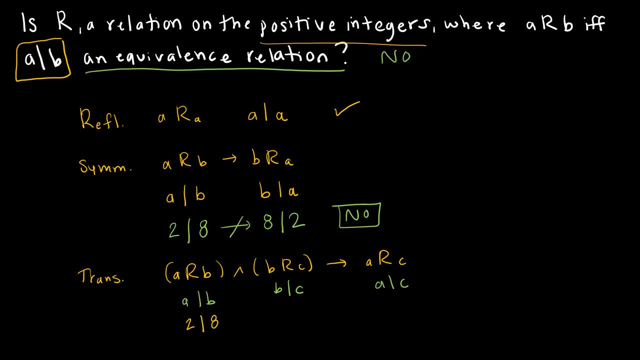 So 2 divides Divides 8.. We already know that's true. 2 goes into 8 four times 8 divides 16.. So again these two. it's a given that they're true. So 2 divides 8.. 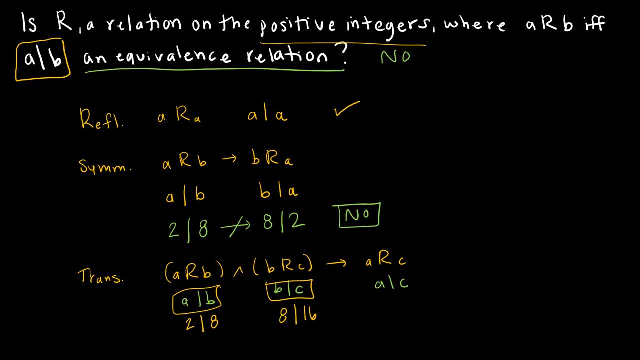 8 divides 16.. That's totally true. A divides C is 2 divides 16.. And the question is: is that true? Is it always going to be true, and not just true for the example that I made up? And it is always going to be true. 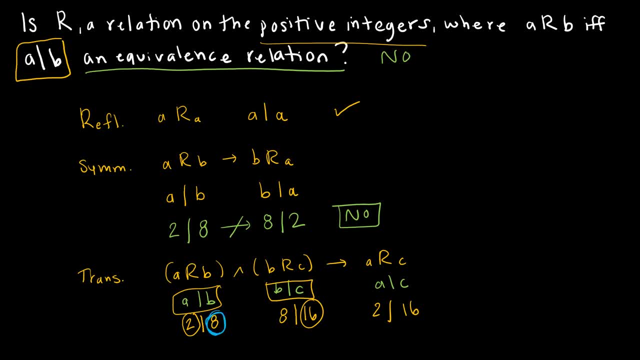 Because if 2 goes into this number and this number is just a multiple of this number, then it's always going to be true Every single time. So yes, this in fact is transitive. Is it an equivalence relation? 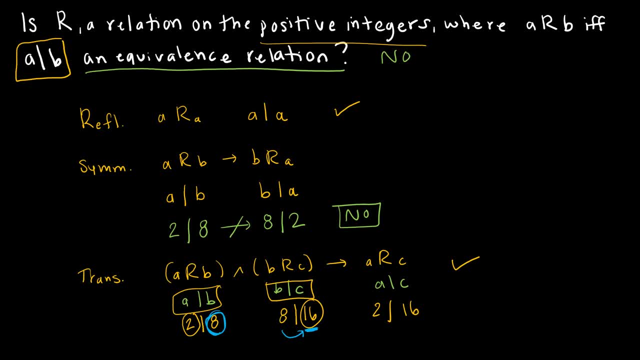 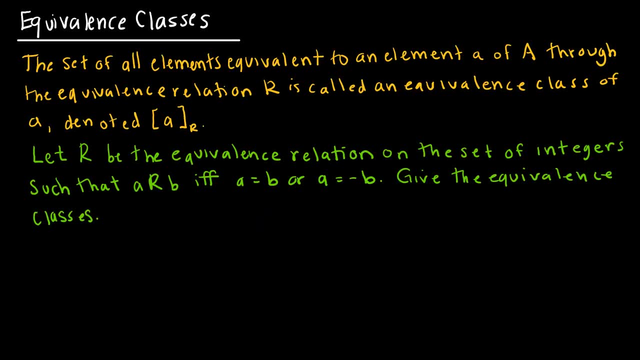 No, because it is not symmetric, But it is reflexive and transitive. Often, when we are talking about equivalence relations, we talk about equivalence classes, And an equivalence class is essentially just a grouping Or a set of all elements that are related through a relation. 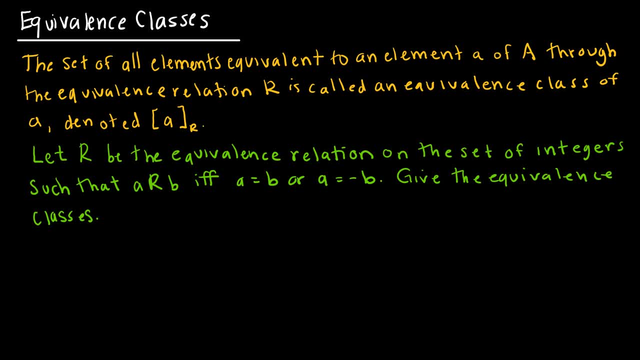 So, for instance, if R is the equivalence relation on the set of integers, such that A is related to B, If, and only if, A equals B or A equals negative B, And they want us to give the equivalence classes, So let's think about what would happen here. 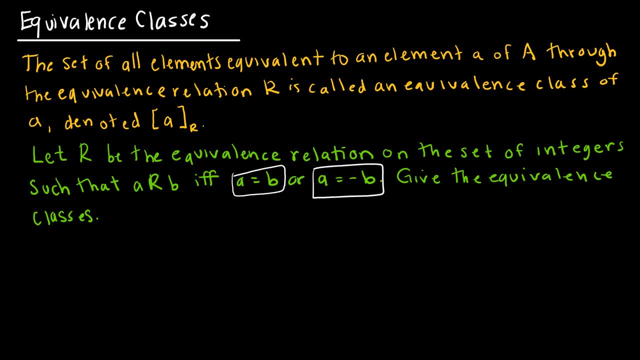 If I'm taking A equal B and A equal negative B, then things that would be related is: 1 is related to itself And also related to negative 1. These things would be grouped together. Zero would be obviously just related to itself. 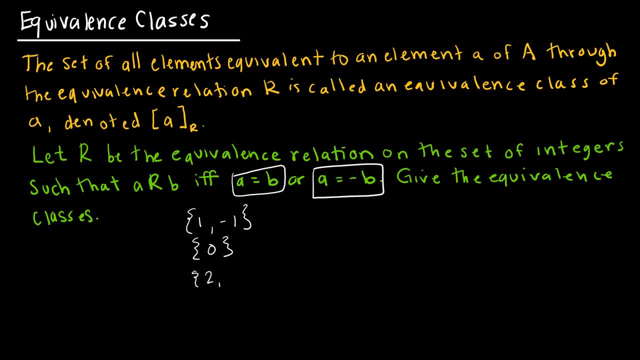 There would be no negative value. The value of 2 would be related to the value of negative 2. Because that would be A equals B or A equals negative B And 3 would be related to negative 3. And you get the idea. 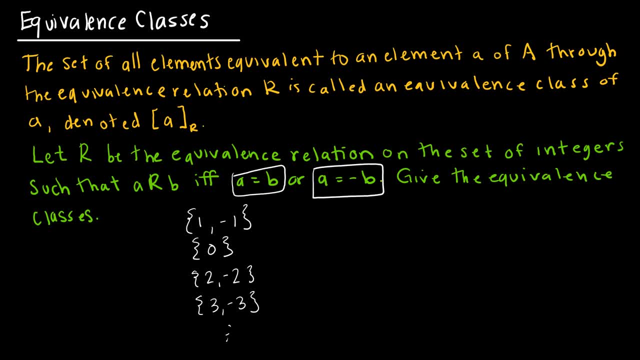 Now it's impossible for us to list all of these. So essentially, what we do Is we use this notation and we say: let's just choose a representative, And obviously it's easier to choose a positive representative. 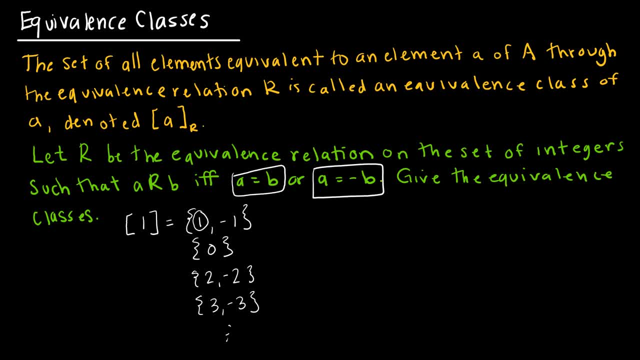 So I'm choosing the representative of 1 for the equivalence class And an equivalence class of 0. And an equivalence class of 2.. And again, all I'm doing is saying all of these values within that equivalence class are related. 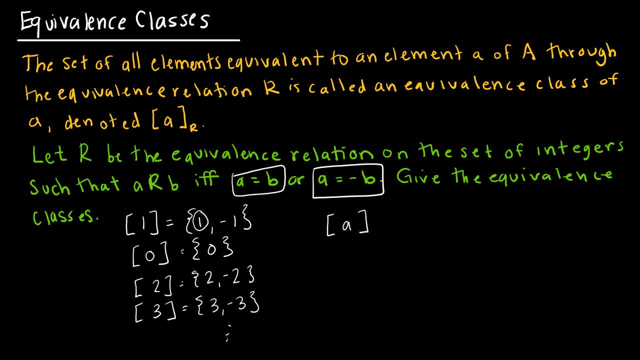 And so, to make this easier, I would say that A Would equal B And A equals B, Include both the positive A value and the opposite A value. So if the original A was negative, then the other one would be a negative negative, which is positive. 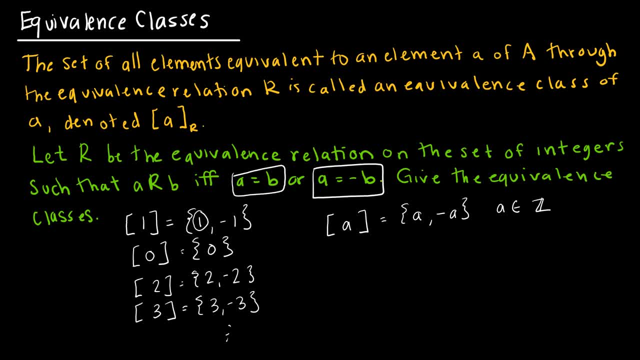 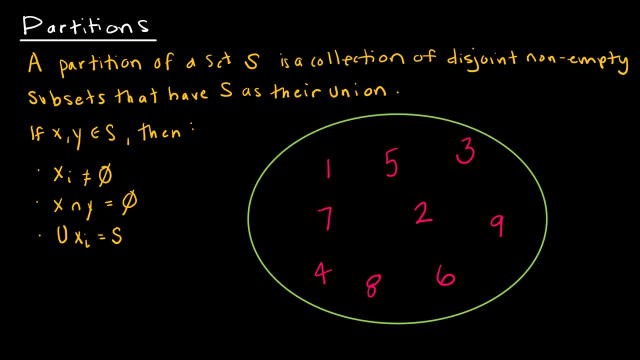 We get the idea Where, of course, A is an integer. So this would be an easy way to generalize that. But again, the equivalence class just relates things that, basically that are related through the equivalence relation. Let's take a look at a partition example. 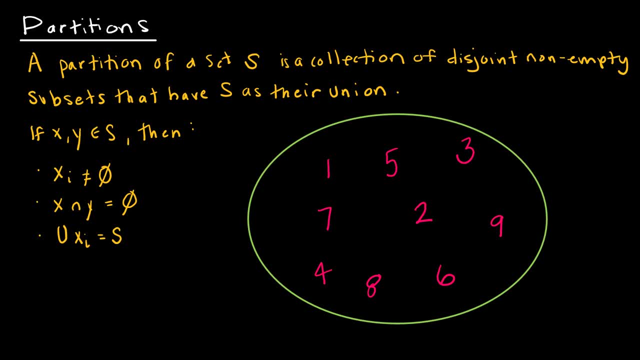 And partitions are great to help us to understand equivalence relations. But first, before we look at an equivalence relation, let's just look at what a partition is, in case you've never encountered one before. A partition of a set S is a collection of disjoint, nonempty subsets that have S as their union. 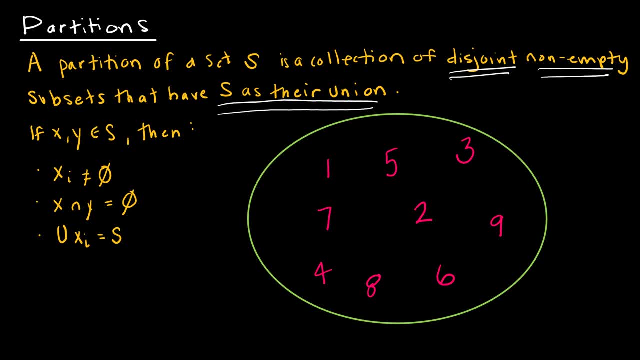 So that's our conditions: Disjoint, nonempty subsets that have S as their union. So what does all of that mean? We're saying that if Xi is some subset, that it's not empty Nonempty subset. They are disjoint, which means their intersection is the empty set, which essentially means when I partition these values, I can't have an element that's in more than one subset. 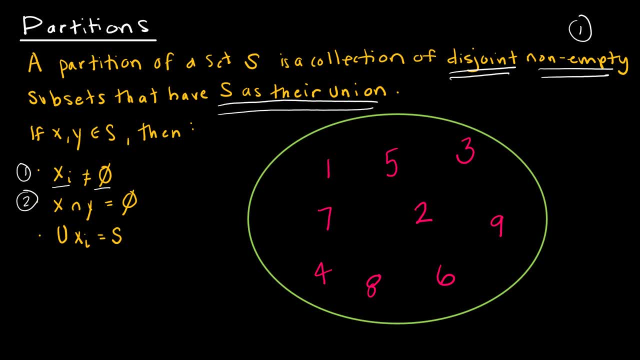 And then, of course, they have S as their union. So the union of all of the subsets is equal to the set, which means I didn't leave anything out, and if I add all of the subsets together, I get the original set. 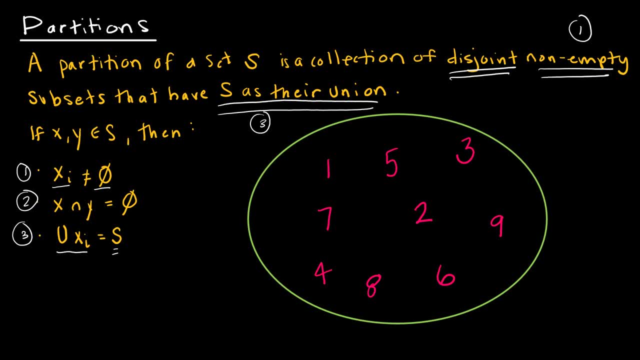 So let's look at how I could possibly partition the digits 1 through 9.. I could just randomly partition them. This would be considered a partition. Let's call this A1, A2, A3.. Was there any rhyme or reason to how I partition these? 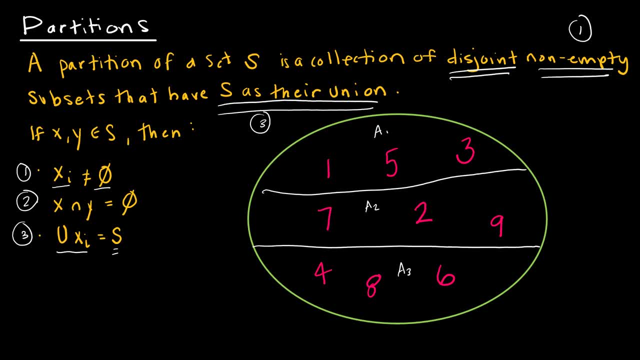 No, but does it fit the bill in terms of a partition? Are these disjoint? Yes, because there is not an element in A1, that's in A2 or A3, etc. Are these nonempty? Yes, each element or each subset- A1,, A2,, A3, all has at least one element. 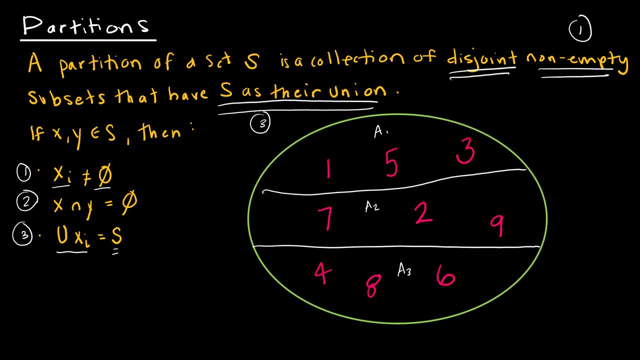 And do they have S as their union? Yes, all of the elements that were contained in my green circle of digits, 1 through 9, are all accounted for in one of the subsets, So this is a valid partition. Let's take a look at another that maybe has some reasoning behind it. 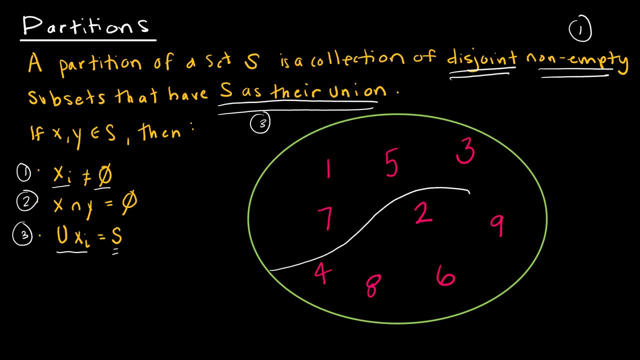 What if I wanted all of my even values to be together? So I have 2,, 4,, 6,, 8.. We'll call that A1.. And 1,, 3,, 5,, 7,, 9.. We'll call that A2.. 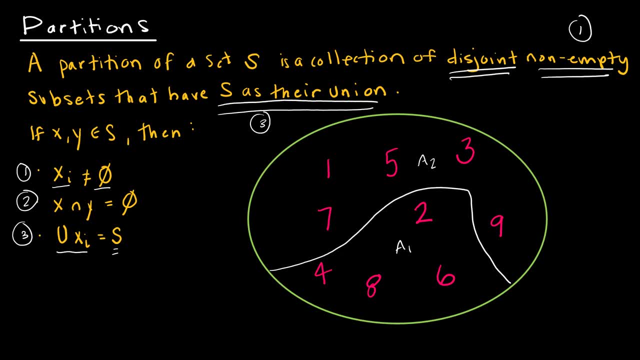 So, again, this is a great way to partition them as well. Let's look at one related to discrete math, since that's what we're studying. What if I looked at division mod 3?? Well, mod 3,, if you'll recall, has everything to do with what is the remainder when I divide by 3.. 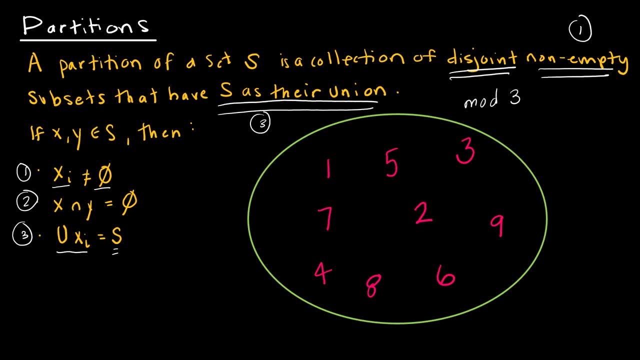 And the only possible remainders when I divide by 3 are 0,, 1, and 2.. I can't have a remainder of 3 because that would just add one more to the quotient. So 0,, 1, and 2 are my possible remainders. 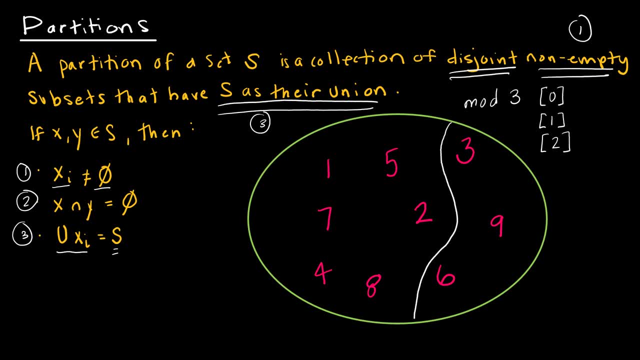 So if I grouped 3,, 6, and 9 together, any of those divided by 3 has a remainder of 0. So those are the elements that belong to my equivalence class And again note the notation. 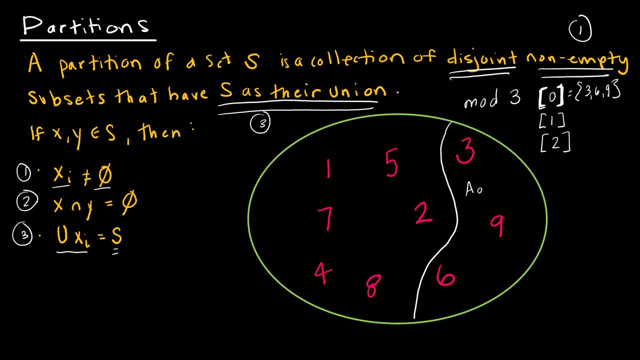 I've got the brackets around the 0. And I chose 0 because that is the remainder. So what about 1, 4, 7?? Well, if I divide 1 by 3, I get 0, remainder 1.. 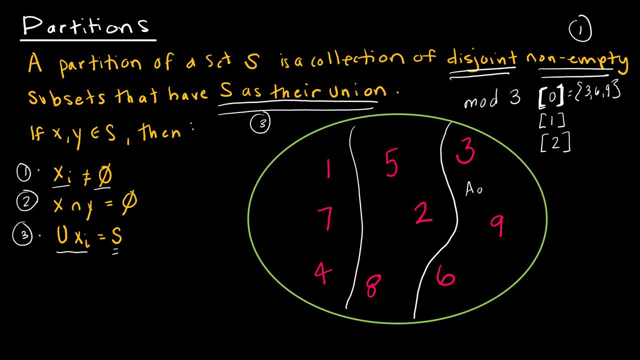 If I divide 4 by 3,, I get 1, remainder 1.. And if I divide 7 by 3,, I get 2, remainder 1.. So this is my equivalence class for a remainder of 1, which is 1,, 4,, 7.. 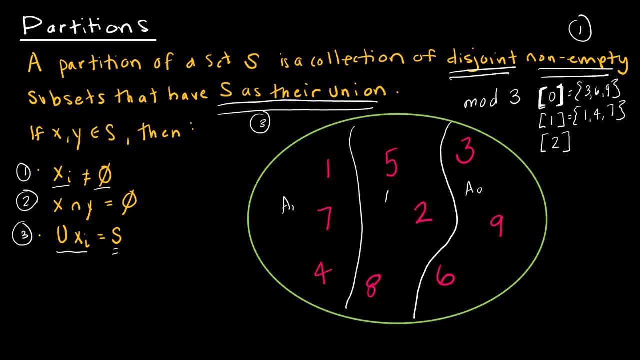 And then again 2,, 5, and 8 all have a remainder of 2.. So the equivalence class for 2 is 2, 5, 8.. So again, I've chosen some representative for the name or label for my equivalence class. 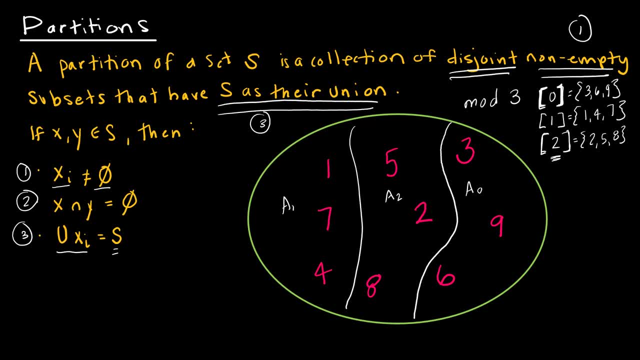 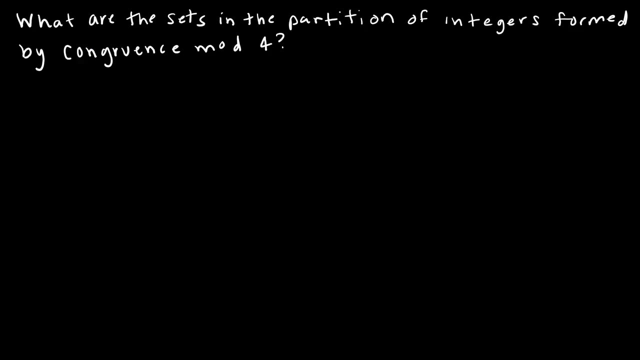 But that is a valid partition because, again, no empty subsets, the intersection, there's no overlap. If I add up all of the subsets, they do add up to the set itself. Let's take a look at another example now, And this is similar to the last one. 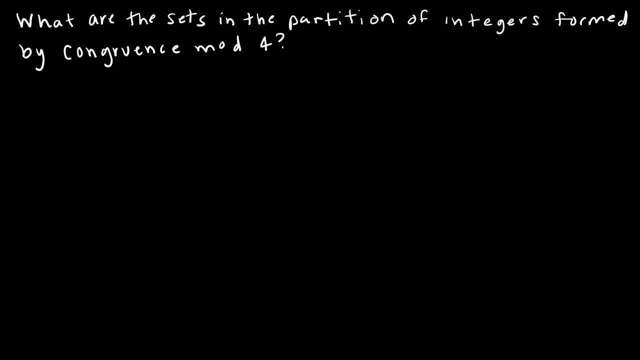 In the last example, we did mod 3.. However, we only had 9 digits to deal with, And now I'm asking for the partition of integers. So obviously there's going to be more values, But it's the same concept. 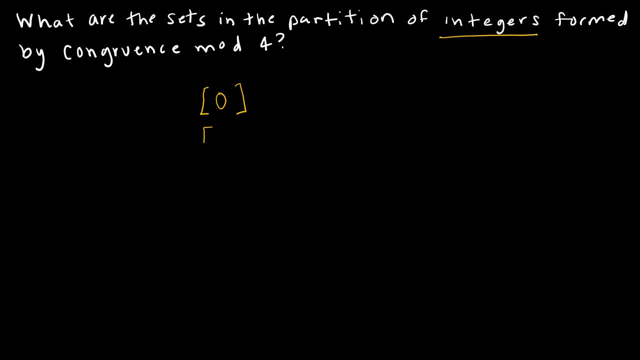 I can either have a remainder of 0 or of 1, or of 2 or of 3.. And so essentially, what they're saying is: give me the values that belong to the equivalence class of 0.. So we know the values in the equivalence class of 0. 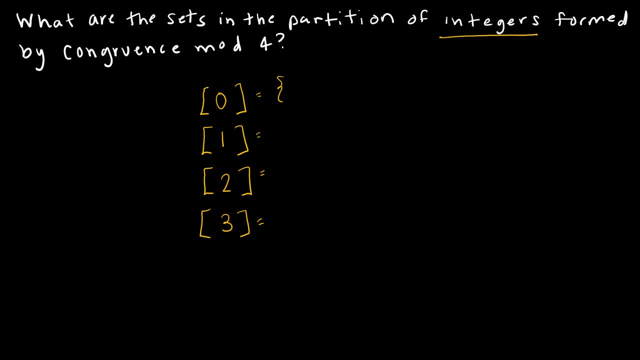 would be things that are divisible by 4 evenly, So 0 is divisible by 4 evenly, And 4 and 8.. And this would continue on forever in the positive direction: Or negative 4, or negative 8, or negative 12.. 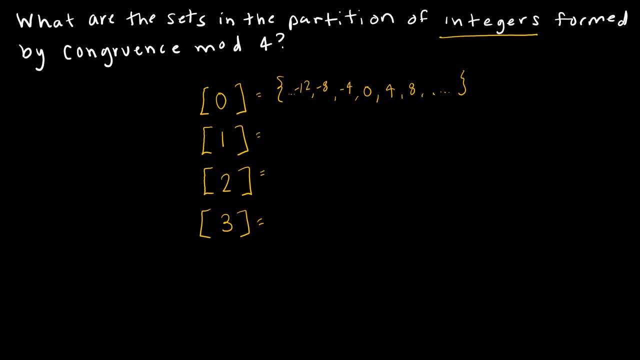 And it would continue forever in the negative direction. So that's how I might write that for the equivalence class of 0.. Now let's look at the equivalence class for 1.. So I know for sure that 1 has a remainder of 1. 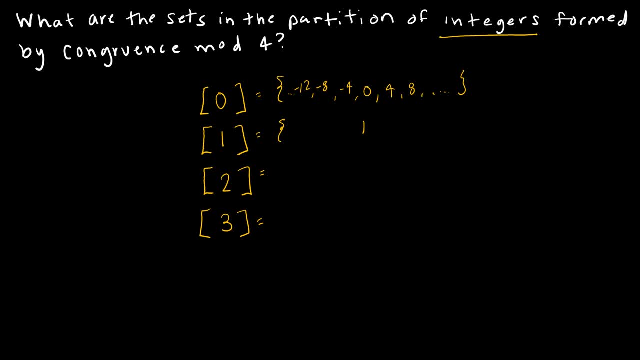 because 4 goes into 1, 0 times with a remainder of 1.. And essentially I'm just going to add 4 and add 4 and add 4.. And then I'm going to subtract 4 and subtract 4.. 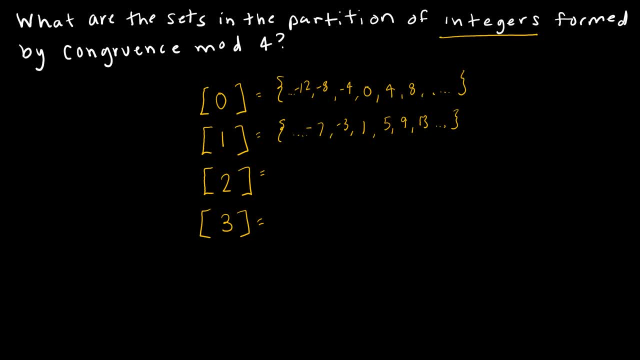 And know that it goes forever in each direction And I'm going to continue that process. So 2, obviously, And then I'm going to add 4 and add 4.. Or I'm going to subtract 4 and subtract 4.. 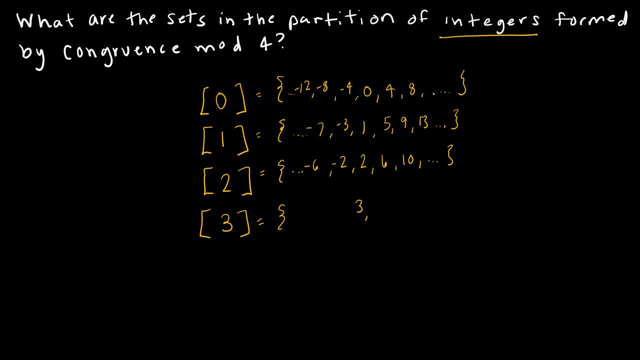 And then for 3, obviously 3 works, And I can add 4 and add 4.. Or I can subtract 4 and subtract 4.. Oof, try that again. 1 minus 4 is negative 5.. 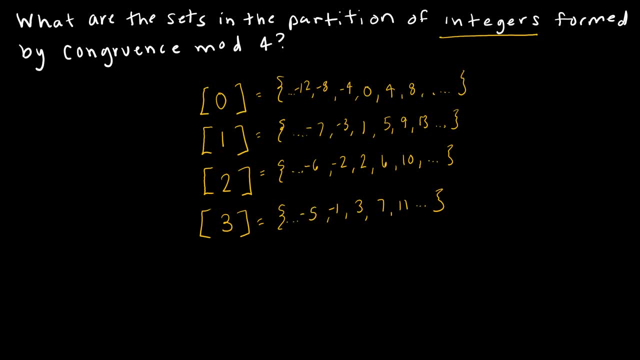 There we go Now. the question then is: is this a partition? So do I have any empty subsets? No. Do I have any overlap in my equivalence classes? No, I don't. If I added up all of these in here. 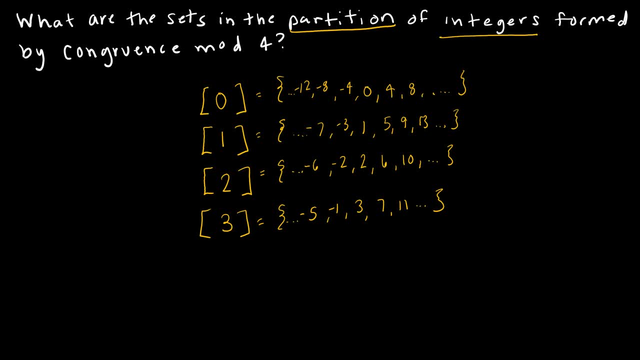 is it the set of all integers? And yes, it is So: 0,, 1,, 2,, 3,, 4,, 5,, 6,, 7,, etc. And then, of course, on the negative side, 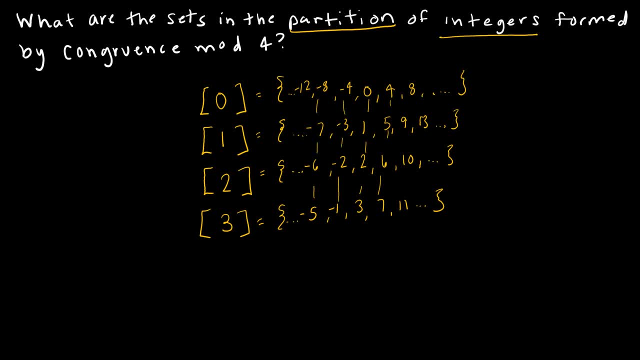 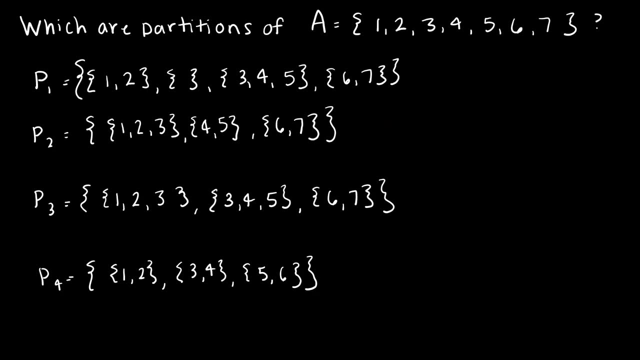 negative 1, negative 2, negative 3, negative 4.. And it continues forever. So, yes, this is a partition And, again, these are the equivalence classes based on that partition. We're going to end with 4 examples or non-examples. 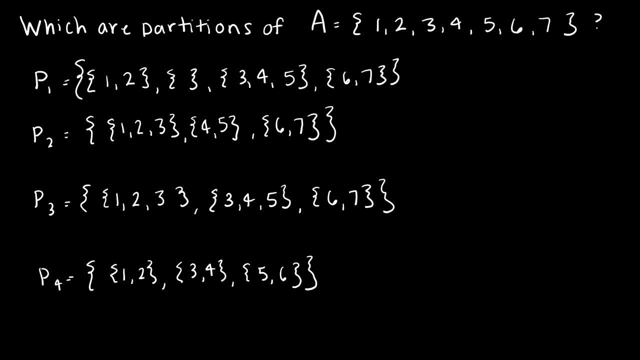 Essentially, we're going to look at these 4 partitions and say: are they in fact partitions? And so, if you'll recall, in order for them to be partitions, we need no empty set, We need no overlap And, again, that's not the official mathematical term. 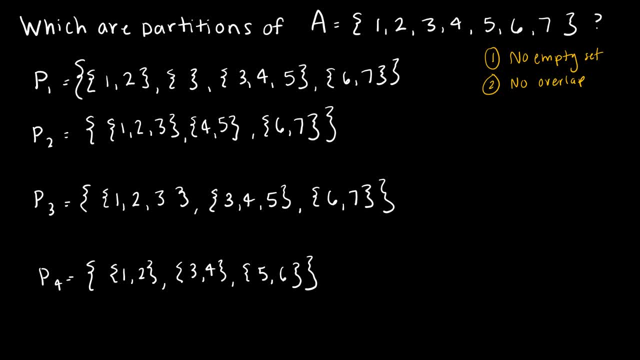 We're saying that the intersection of the sets must be the empty set, But essentially that means no overlap And is the union, the entire set, So all elements included. So these are the things that I'm going to check for, each of these possibilities. 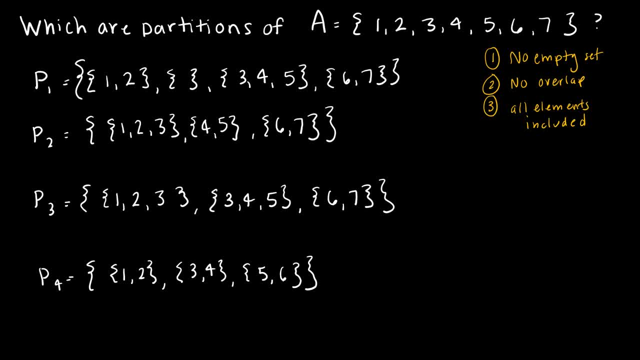 And I'm just going to write a yes or a no next to them, whether they are partitioned or not. So for the first one- P1,, we're saying we have the subset 1, 2.. We have the subset 3,, 4, 5.. 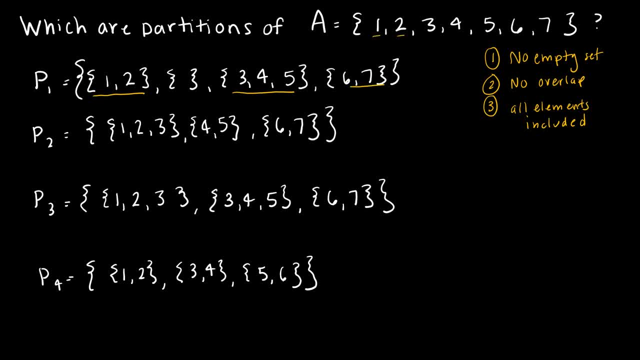 And we have the subset 6, 7.. And looking at 1,, 2,, 3,, 4,, 5,, 6, 7, yes, all elements are included. There is no overlap, which means I didn't use any of those values more than once.